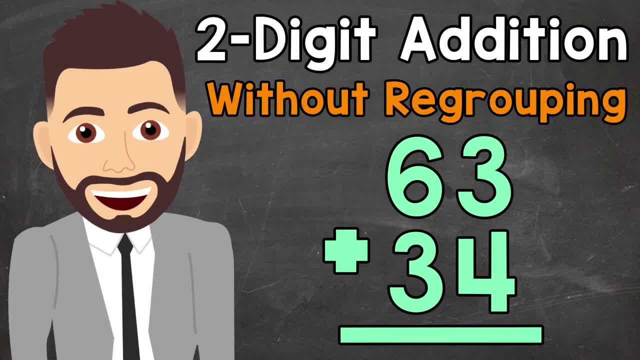 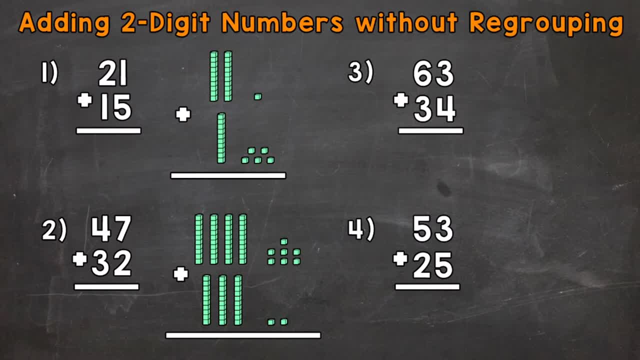 Welcome to Math with Mr J. In this video, I'm going to cover how to add two-digit numbers without regrouping, and we have four examples that we're going to go through together in order to get this down. So let's jump into number one, where we have 21 plus 15.. Now I have some base 10. 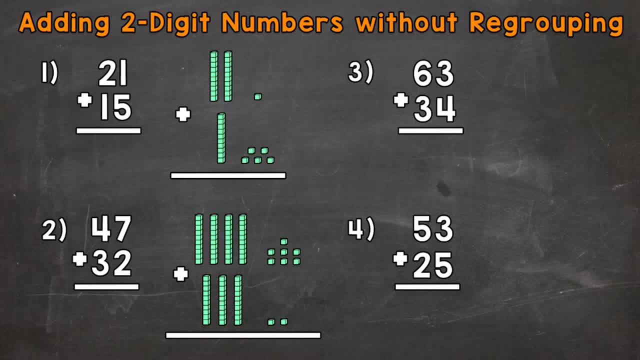 or place value blocks to the right. That's going to help us visualize exactly what's going on throughout this problem. So we always start with the ones place when we add. So we need to do one plus five. We have one one plus five ones, So that's going to give us a total of six ones. 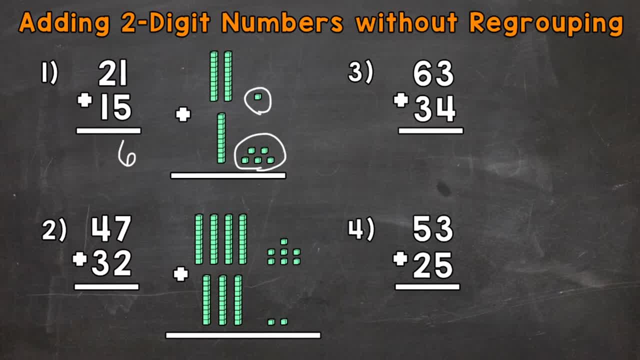 One plus five is six Now we do the tens. So for 21, we have two tens and for 15, we have one ten. So two tens Plus one ten gives us a total of three tens. Two plus one is three, Now that three represents. 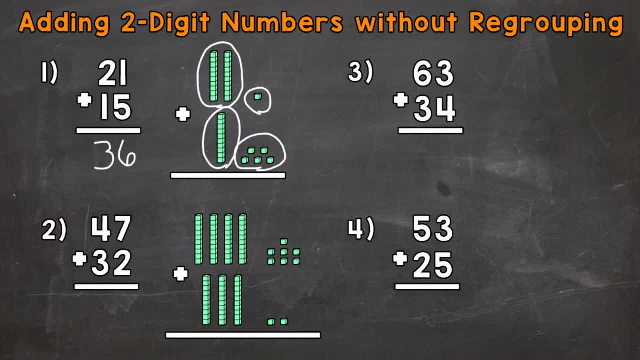 30, three groups of 10.. So our final answer there is 36.. Let's go on to number two, where we have 47 plus 32.. So again, always start with our ones. So seven ones plus two ones. 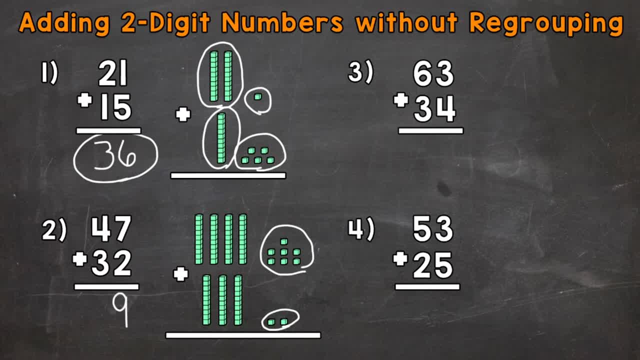 gives us a total of nine ones. Now to the tens. So four tens plus three tens. Again, four tens plus three tens gives us a total of seven tens. Now that seven has a value of 70, because it represents seven groups of 10.. And our final answer is 79.. Let's move on to numbers three. 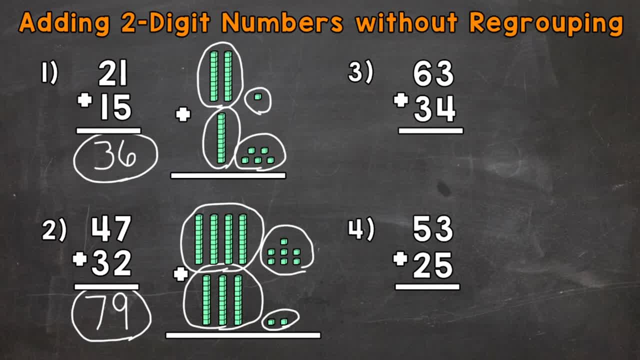 and we're going to do these without the blocks. So for number three, we have 63 plus 34.. Our ones places lined up and our tens places lined up And we start with the ones. So we have three ones plus four ones, That's a total of seven ones. As far as the tens, we have six tens plus three tens. 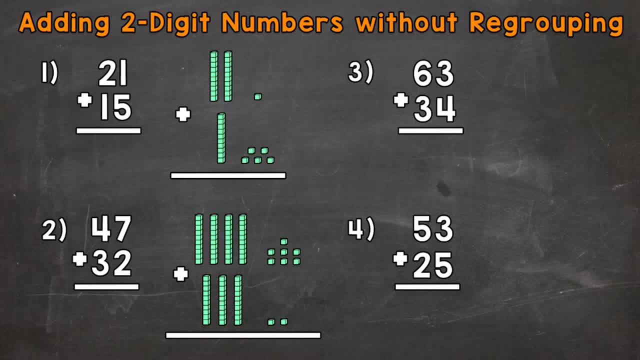 or place value blocks to the right. That's going to help us visualize exactly what's going on throughout this problem. So we always start with the ones place when we add. So we need to do one plus five. We have one one plus five ones, So that's going to give us a total of six ones. 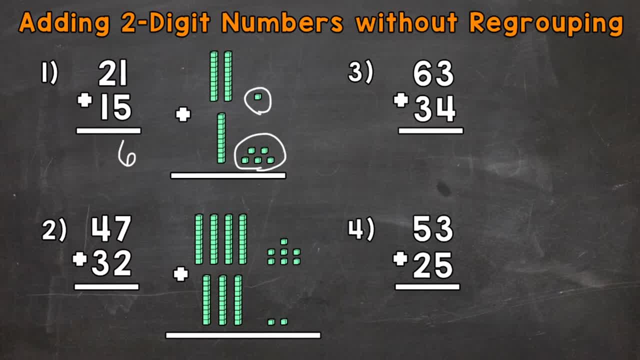 One plus five is six Now we do the tens. So for 21, we have two tens and for 15, we have one ten. So two tens Plus one ten gives us a total of three tens. Two plus one is three, Now that three represents. 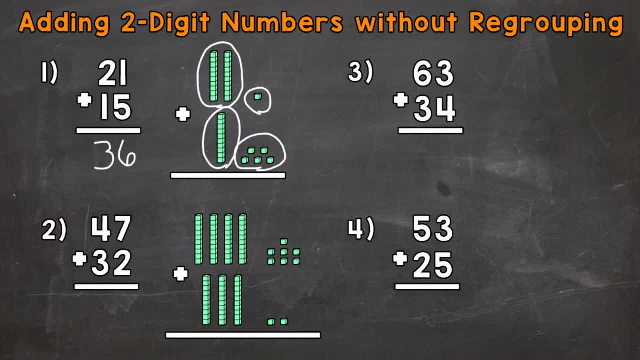 30, three groups of 10.. So our final answer there is 36.. Let's go on to number two, where we have 47 plus 32.. So again, always start with our ones. So seven ones plus two ones. 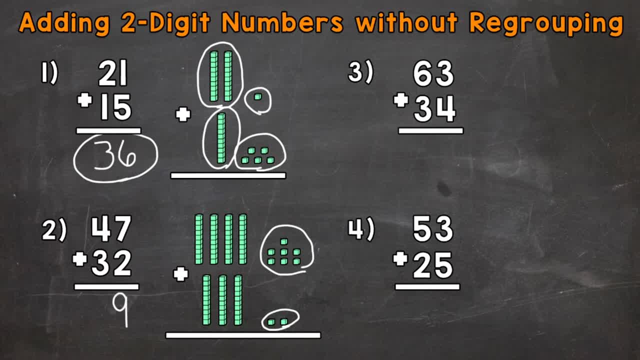 gives us a total of nine ones. Now to the tens. So four tens plus three tens. Again, four tens plus three tens gives us a total of seven tens. Now that seven has a value of 70, because it represents seven groups of 10.. And our final answer is 79.. Let's move on to numbers three. 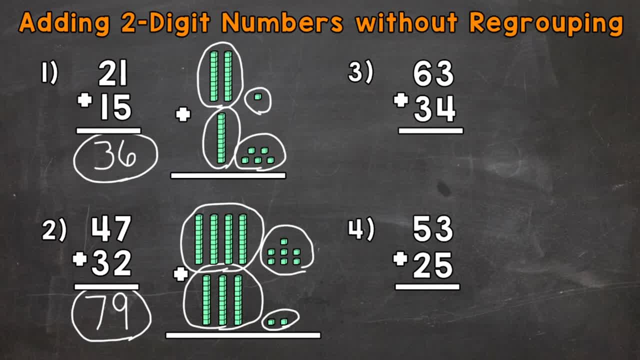 and we're going to do these without the blocks. So for number three, we have 63 plus 34.. Our ones places lined up and our tens places lined up And we start with the ones. So we have three ones plus four ones, That's a total of seven ones. As far as the tens, we have six tens plus three tens. 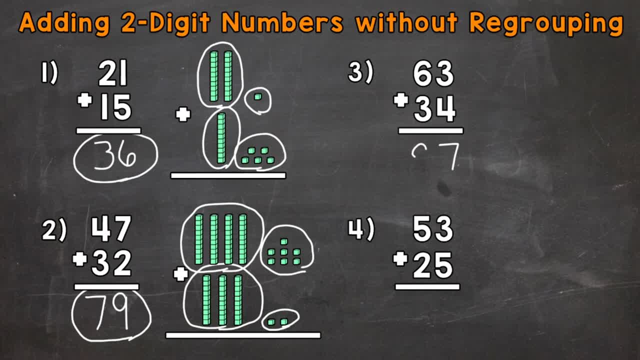 So that's going to be a total of nine tens. Our final answer is 97.. On to number four, where we have 53 plus 25.. So our ones are lined up and our tens are lined up. Start with the ones: Three ones plus five ones. Three plus five gives us eight.